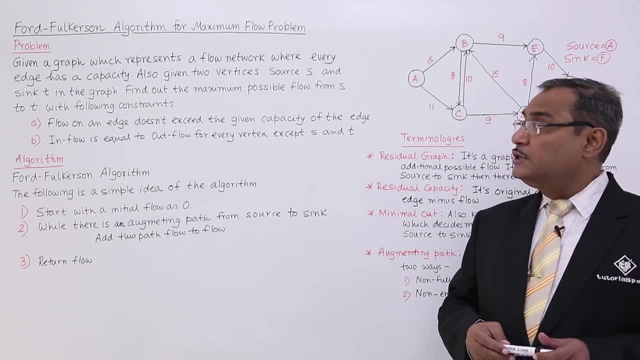 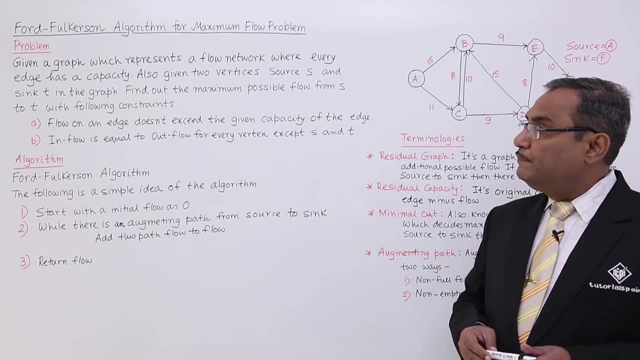 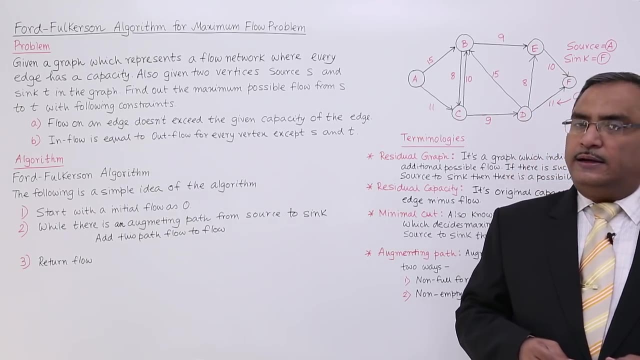 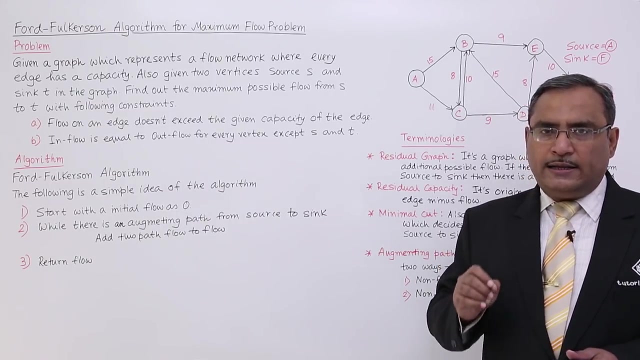 associated, that is the weight of that particular age or branch and that will be denoting the capacity of that age. that means the flow cannot exceed that capacity. also, given two vertices, one is source s and another one is the sink t in the graph, that means the flow will be made originated from source s and will get terminated at sink t. 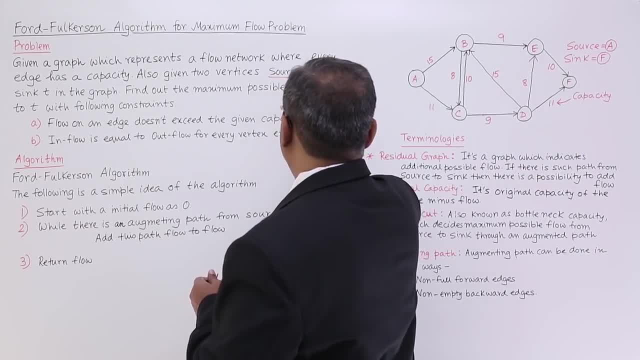 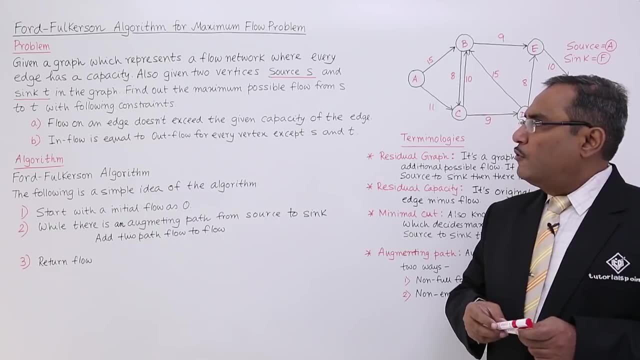 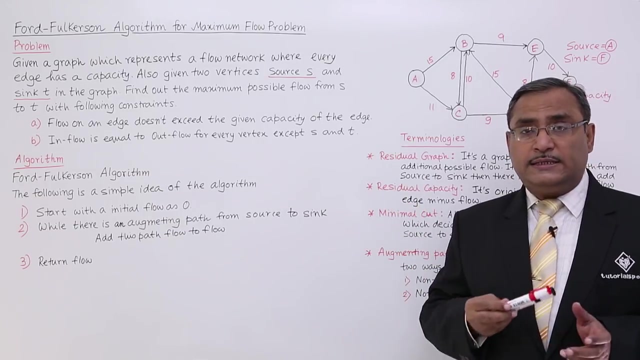 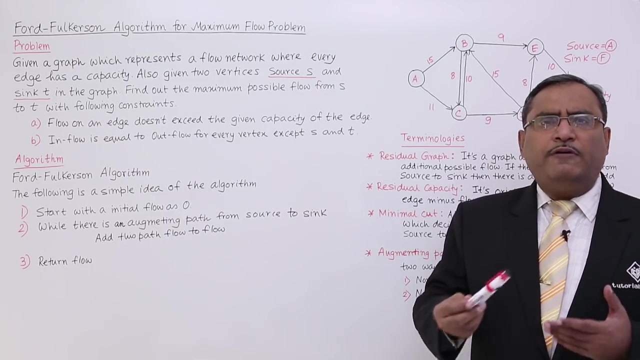 so these are the very important two vertices. are there special type of vertices in the graph? find out the maximum possible flow from s to t with following constraints: so this code fall correction algorithm is nothing but a method which will calculate the maximum flow through our network. here the flow can be of anything. the flow can be of anything. 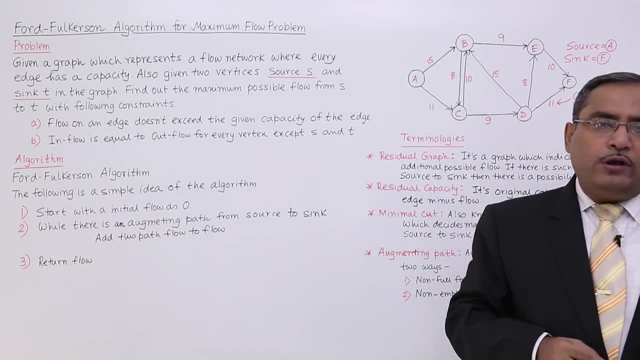 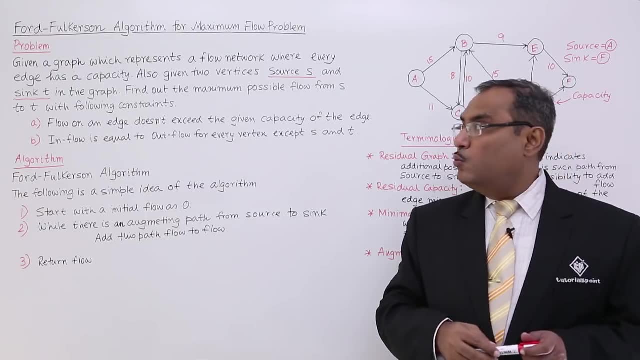 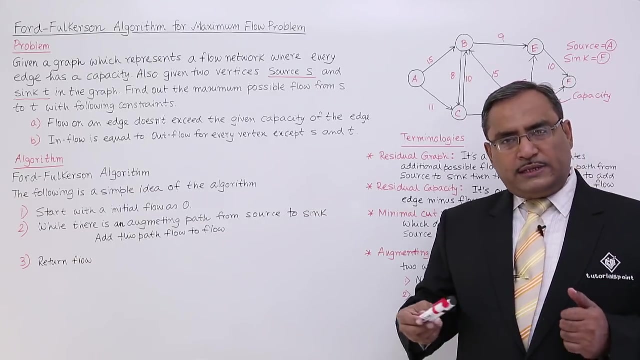 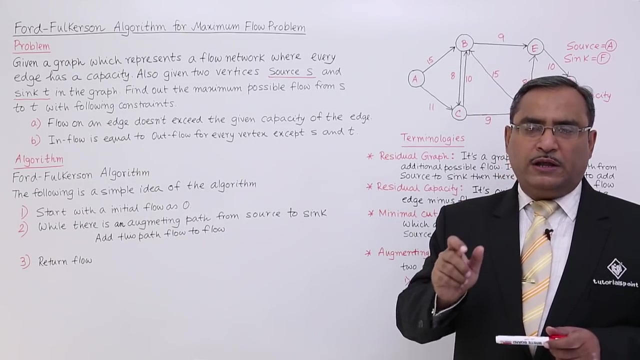 and the maximum possible flow from s to t, with the following constraints. so while calculating the maximum flow through the network, we're having two constants. constant number one: flow on an edge does not exceed that given capacity. obviously, the flow through a certain age should- should not exceed the respective capacity mentioned as an integer value or numeric value. 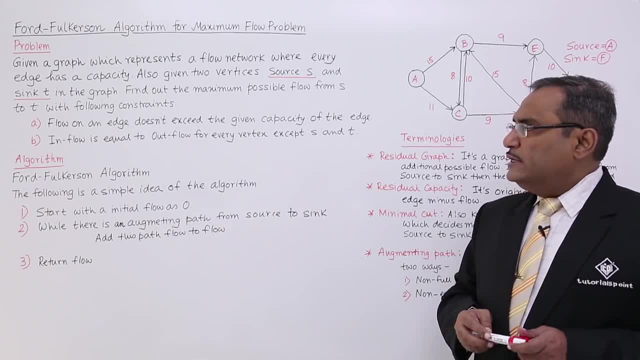 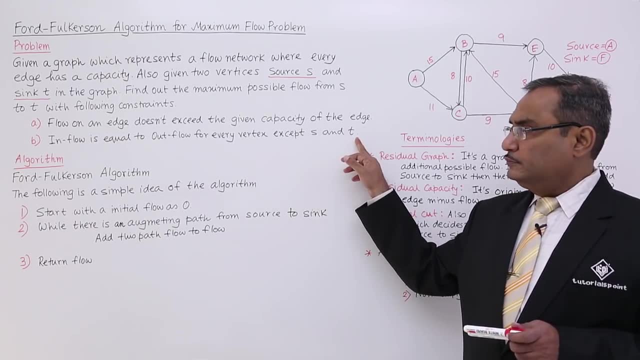 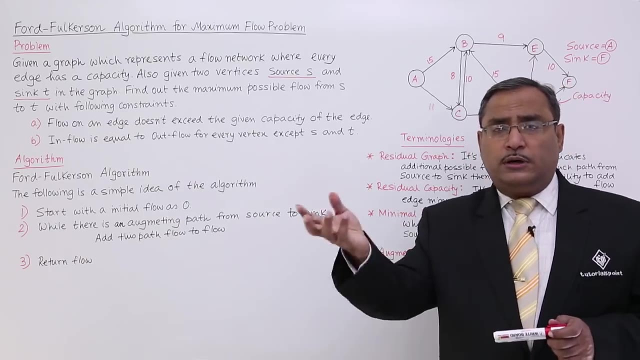 associated with that edge. Inflow is equal to outflow for every vertex except your source and the sink S and T. So obviously the whatever the flow that will come into a vertex should be equal to the flow out from the vertex. But in case of source, only the flow will come out from the source. 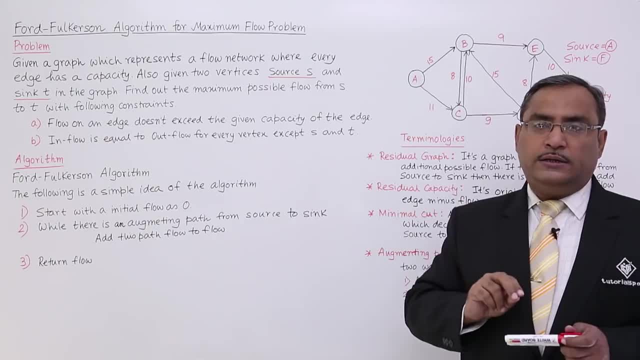 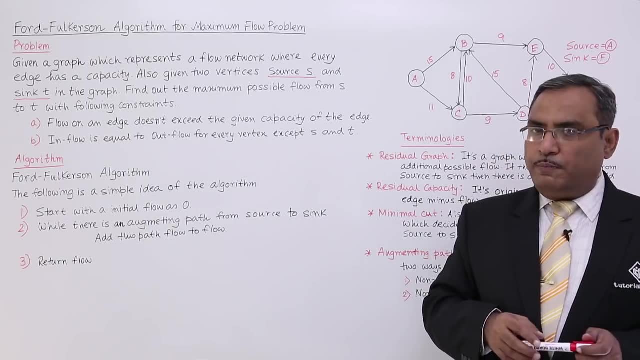 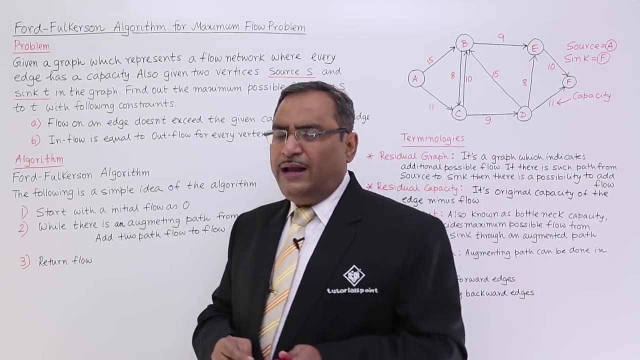 In case of sink T, the flow will go into the sink T, it will not come out. So except these two vertices we are having, the flow in and flow out must remain same in all other remaining vertices in this weighted digraph. So while discussing the algorithm we might be facing different terminologies. 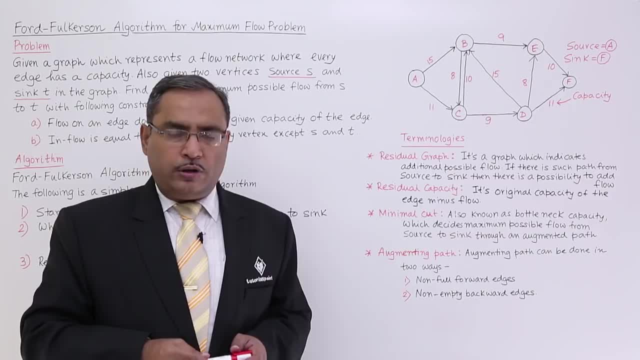 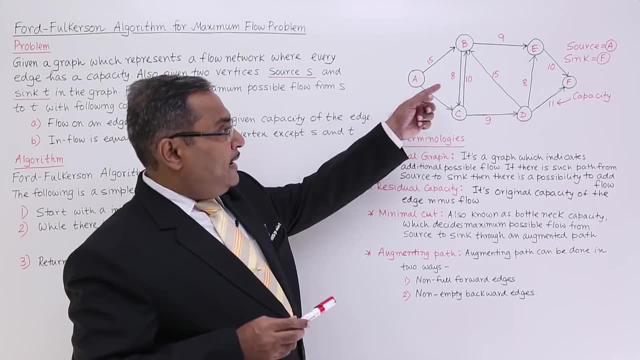 So let me go for the terminologies at first. But before going for the terminology, let us see The. how does one network looks like? you see, these are network. So here: A is the source- we have written that one- and F is the sink or target. 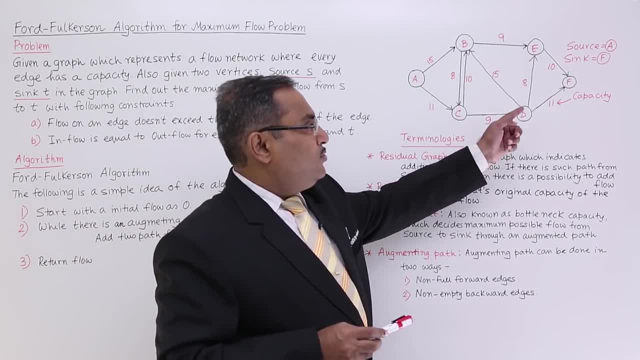 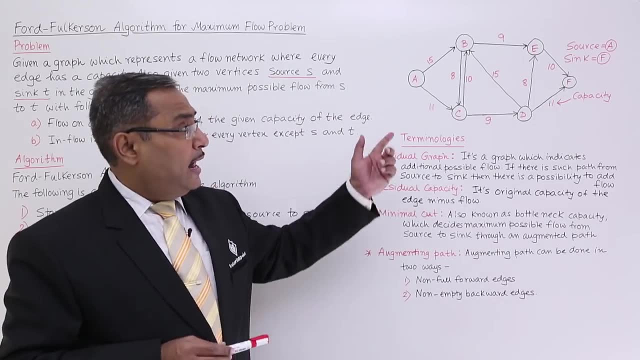 So now, from A, only the flow will come out, and to the sink, only the flow will go in. So these are the respective flows we are having. these are the respective flows we are having and this is a digraph. you are getting this head and tail, for each and every edge. 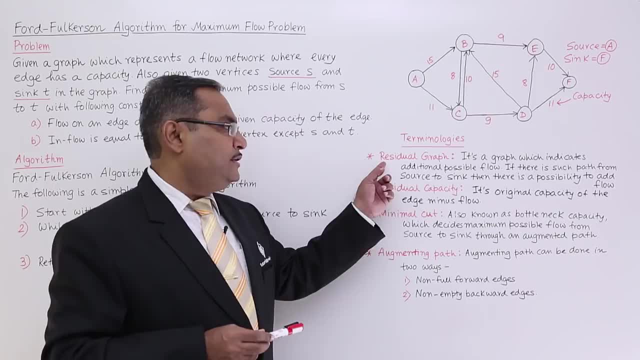 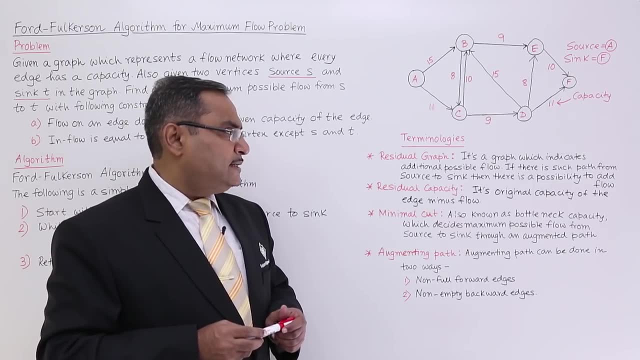 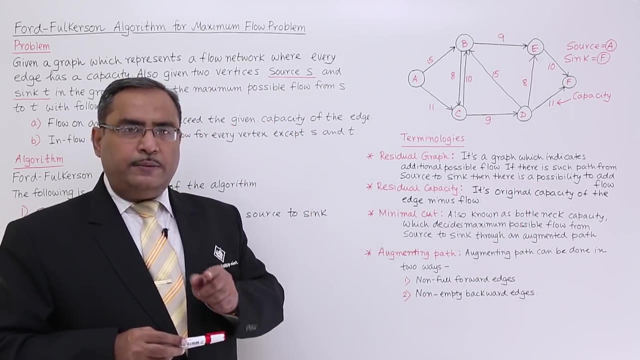 So here are the terminologies. So let me discuss The residual graph. it is a graph which indicates additional possible flow. if there is such path from source to sink, then there is a possibility to add flow. that means through a certain path we can add flow if there is a possibility. possibility means what means the remaining? 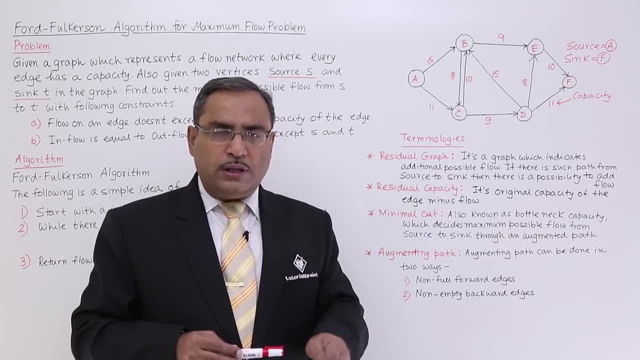 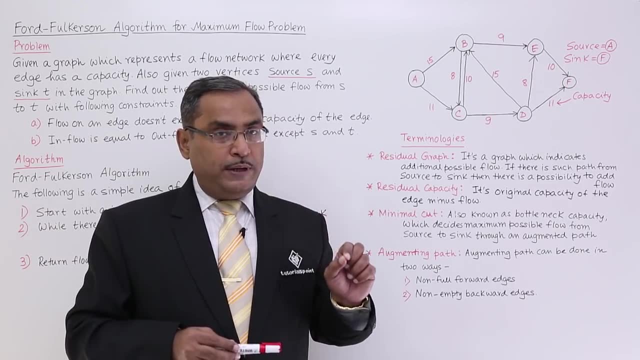 capacity is there and which is non-zero, through the path that is, from the source to the sink, all the edges. So if there is a possibility of falling on the path, they should be having some residual capacity. So let me discuss the residual capacity at first. 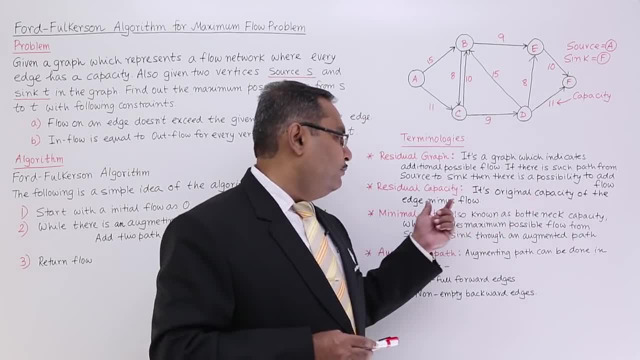 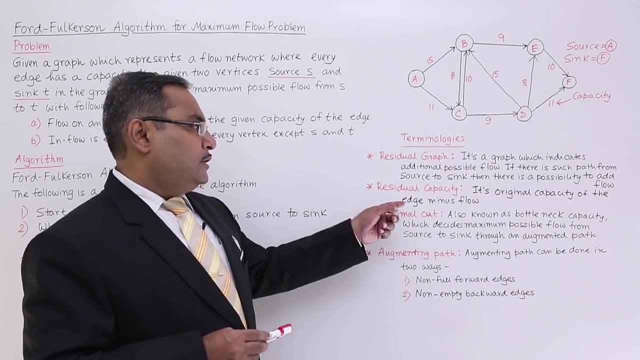 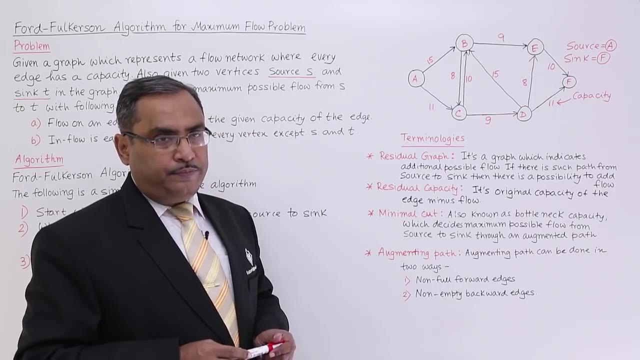 So residual capacity, it is the original capacity of the edge minus the flow. Original capacity means these are the original capacities and minus the flow, So that is known as the residual capacity. Next one is the minimal cut, also known as bottleneck capacity, which decides the maximum. 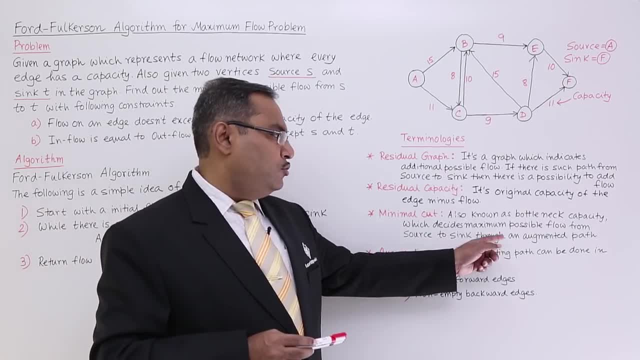 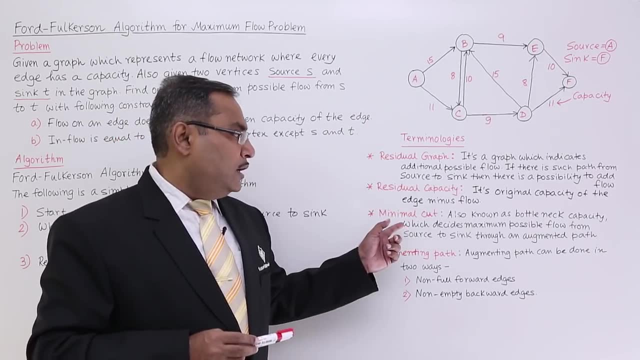 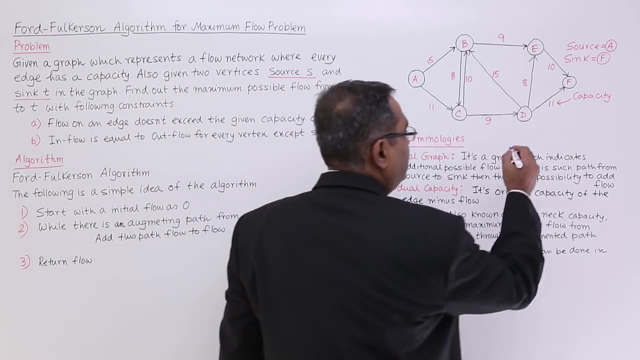 possible flow through From source to sink, From source to sink, through an augmented path. So I think it will be better if we show that one on this particular diagram, what we are trying to discuss through these terminologies. Now see, let us consider we are considering one path, say AC, then D and F, So you are reaching. 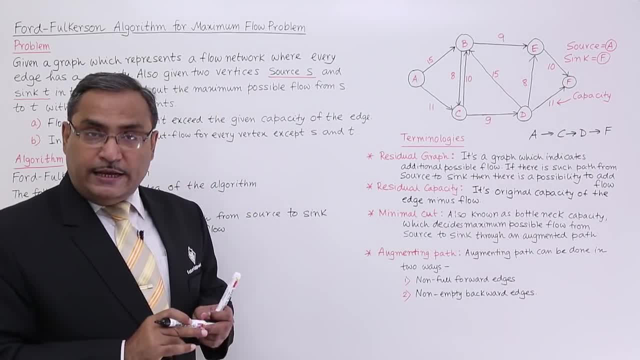 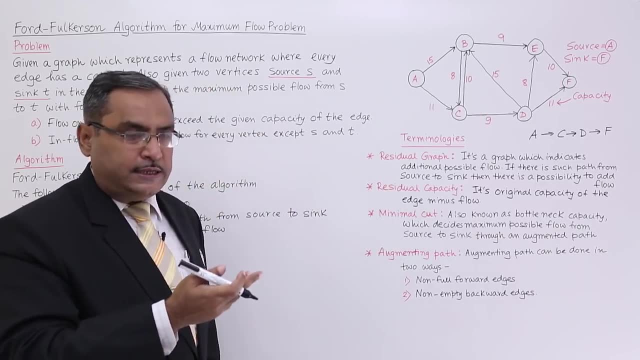 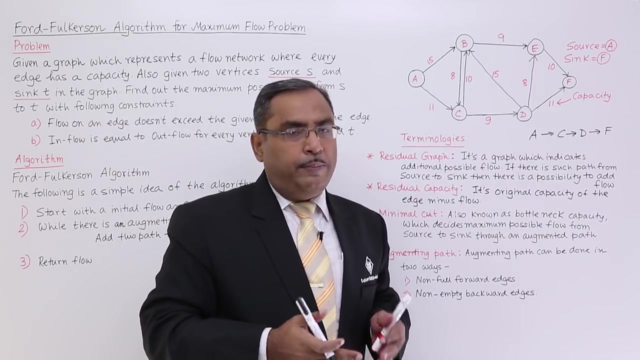 from source to the sink A to F through C and D. Now see, in this particular path the maximum flow is 11. that means the capacity is 11. here the capacity is 9, here the capacity is 11.. So through this path the maximum flow can be 9, because it will decide the maximum flow. 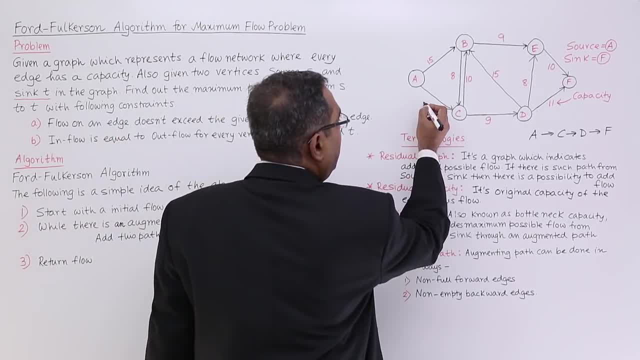 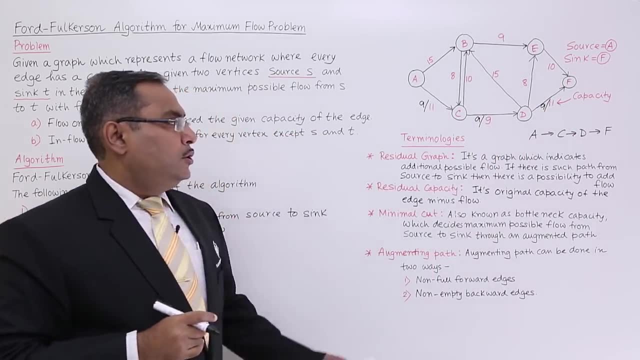 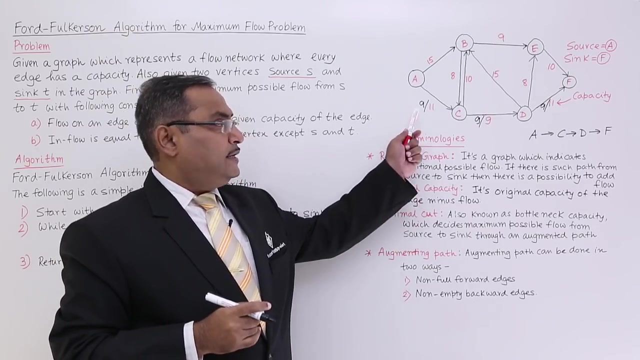 and that is known as the minimal cut. So here I am giving a flow with 9, here 9, and here we are having this. So now see, Now see Here the residual capacity. here the residual capacity is 2, here the residual capacity is: 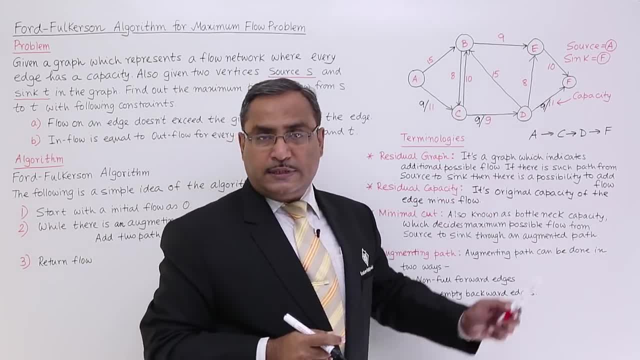 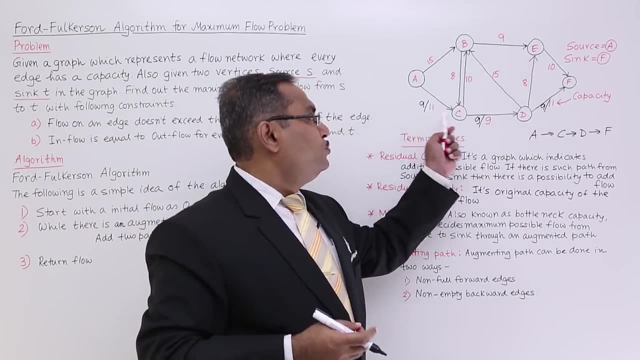 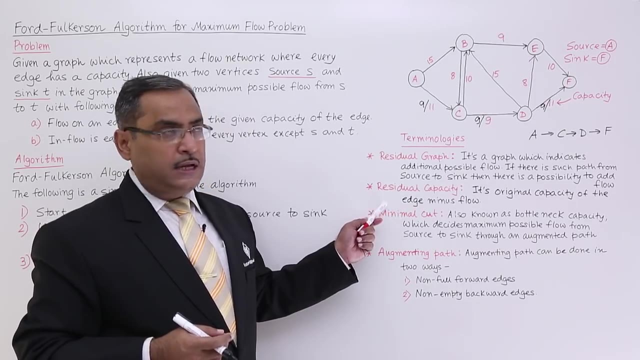 9 minus 9, that is 0. here the residual capacity is capacity minus current flow through that path, through that edge will be 2.. So 2 0, 2 are the residual capacities for the respective edges. So we have discussed what is the residual capacity and the graph thus obtained is known. 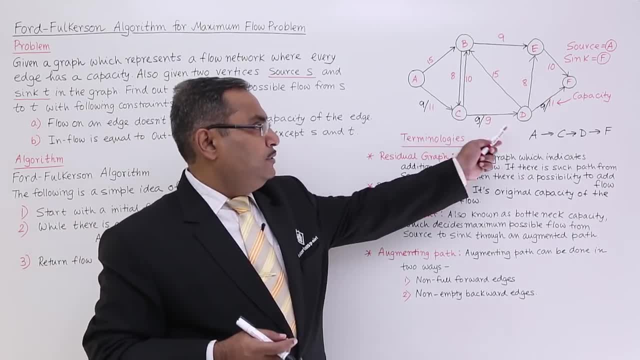 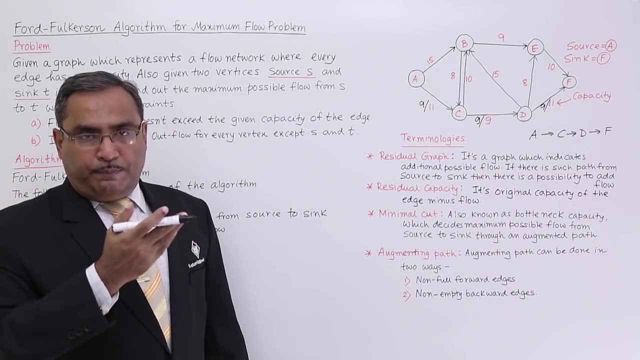 as the residual graph And the minimal cut. I told you this one That is the minimal cut. So minimal cut means the maximum flow possible through that particular path from the source to the sink is the minimal cut. So in this way it is happening. 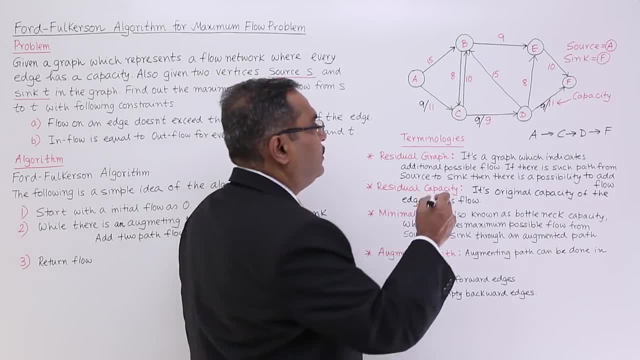 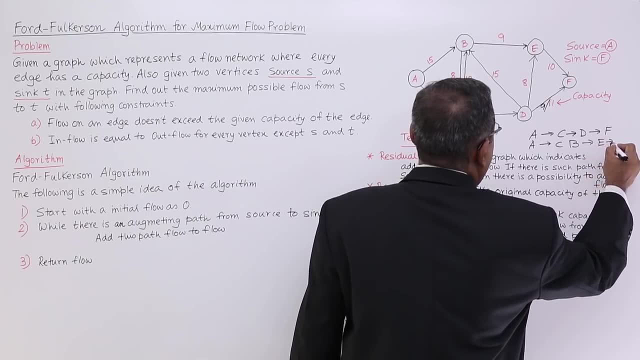 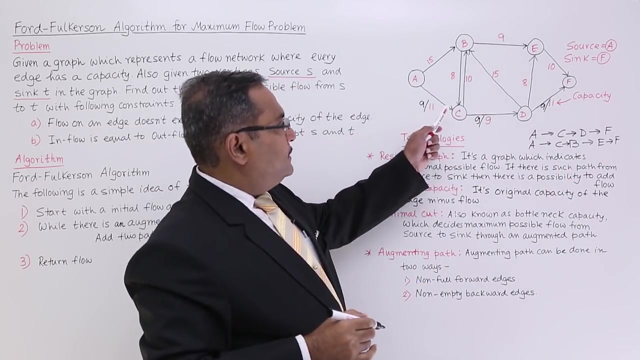 Now see, as it is happening, some capacity there. So if we consider the path, say A, C, B, E and F, If we consider the path like this, So A, C, B, E and F. If we consider the path like this, So A, C, B, E and F. If we consider the path like this: 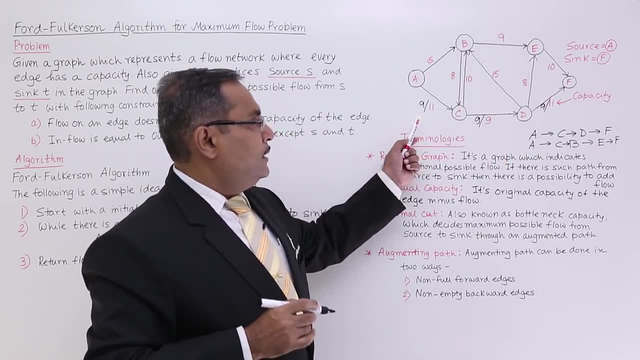 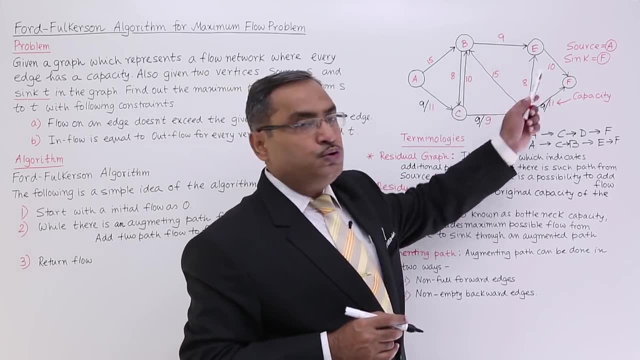 So A, C, B, E and F, Here you see, here the residual capacity is 2.. Here the capacity is 10.. Here the capacity is 9.. Here the capacity is 2.. So that is why we can have the minimal cut here. 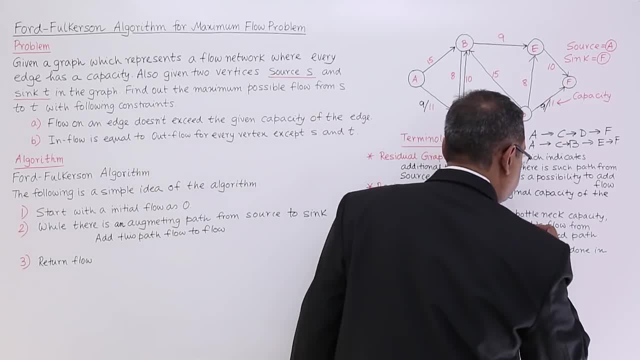 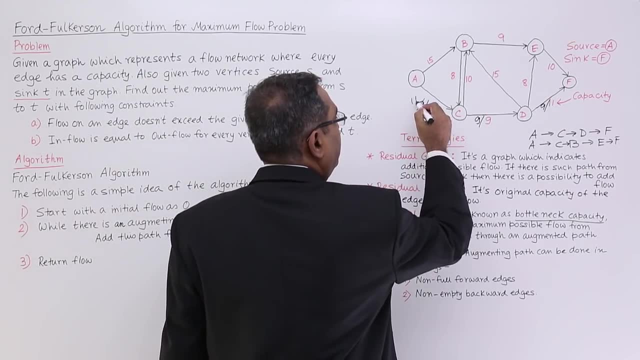 That is a bottleneck. So that is also very important. Bottleneck capacity- this term is very important, So the bottleneck capacity in this particular path is 2.. So what I can do, I can make it 11.. So I can make it 2 there. 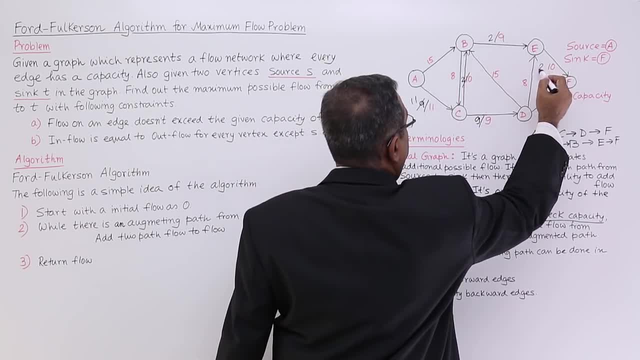 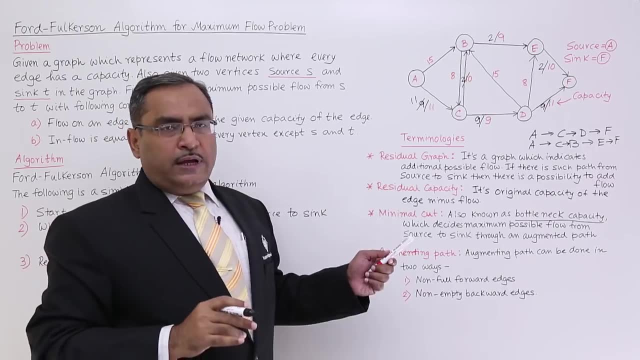 I can make 2 here, I can make 2 here, I can make two here. So here we will be having some residual capacities, but it is quite full In this way. we shall explain in details in the example. Augmenting path can be done in two ways. 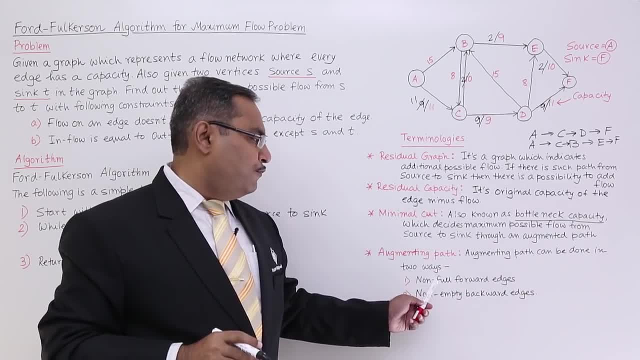 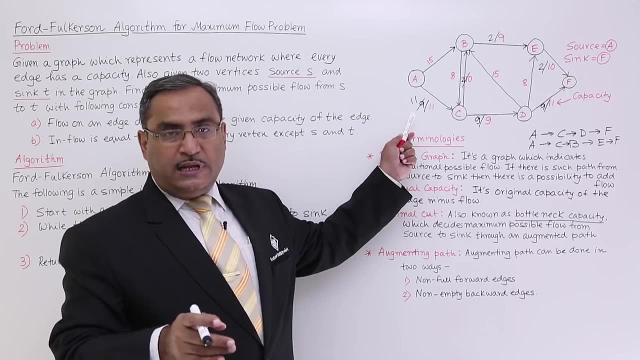 So augmenting path can be done in two ways. One is the non-full forward edges. whatever you have done, It is a non-full. it is a non-full. Initially it was 9 and the capacity was 11. So 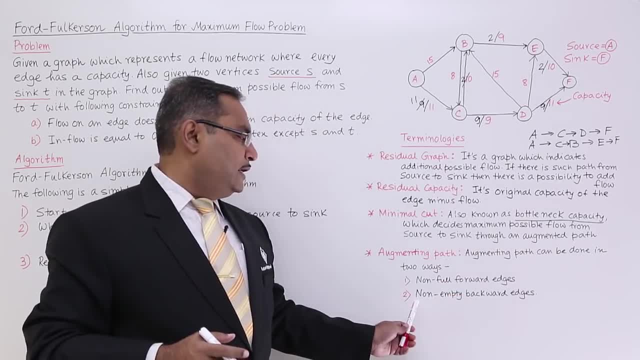 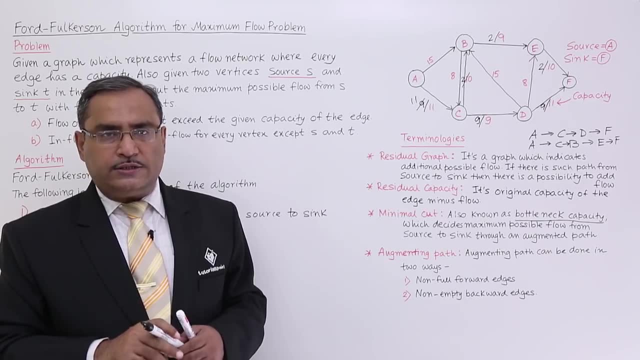 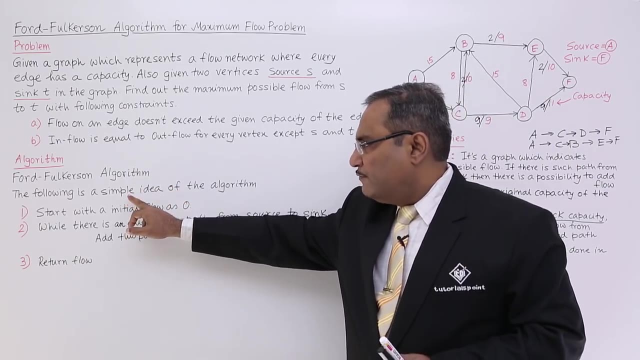 it is non-full, So non-full forward edges, and another one is non-empty backward edges, So non-empty backward edges we shall discuss in one example for the better understanding. So let me discuss the algorithm at first. So Ford-Fulkerson algorithm. The following is a: 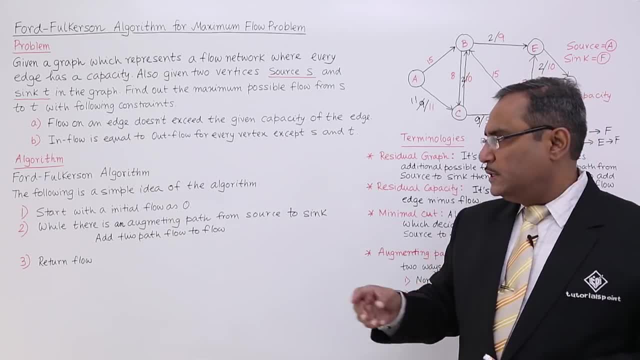 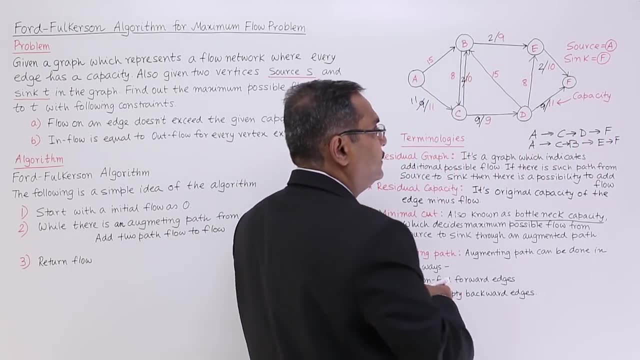 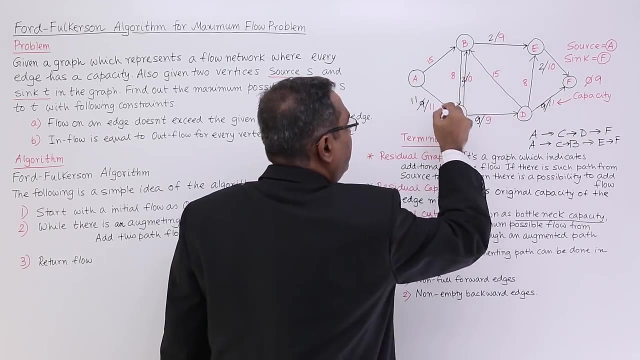 simple idea of the algorithm. We are having three steps. Step number one: start with the initial flow as zero. So initially, I can write here, the flow is zero. Initially, I can write here, the flow was zero. Then we made a flow of 9.. So flow has become 9.. Then we made a flow of 2. 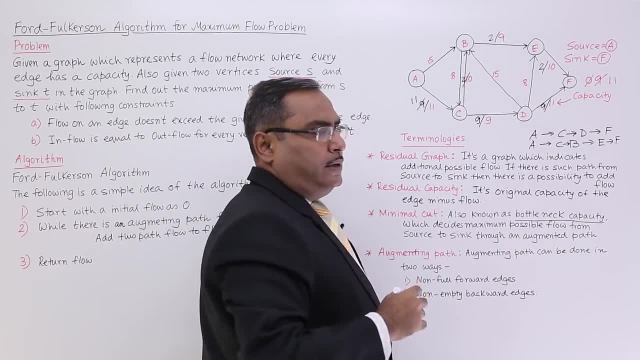 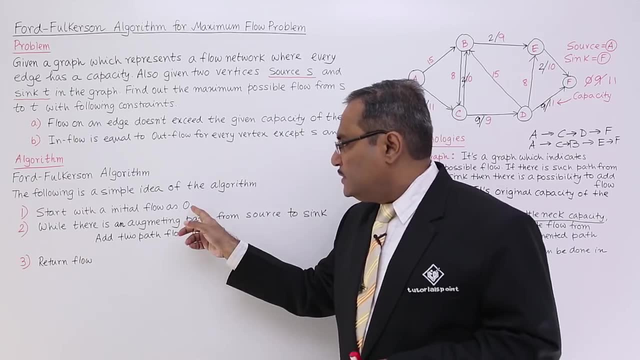 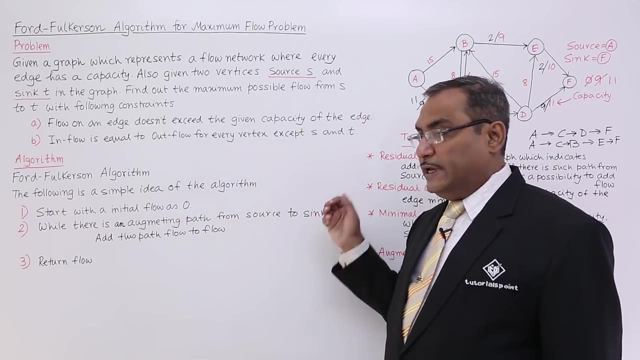 here. So the flow has become 11.. So in this way we will be going for incrementing the flow, because we are going to calculate the maximum flow through the network. So initially we will be starting with the initial flow as zero. Well, there is an augmenting path from source to saying: 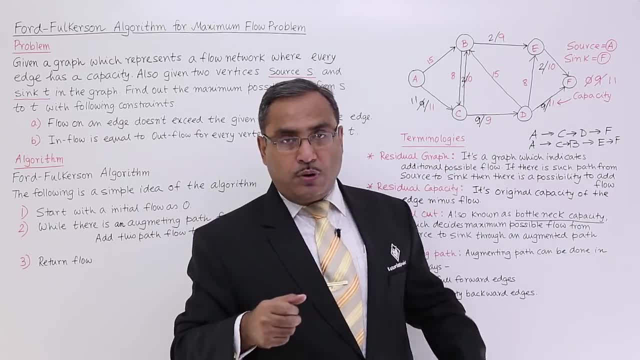 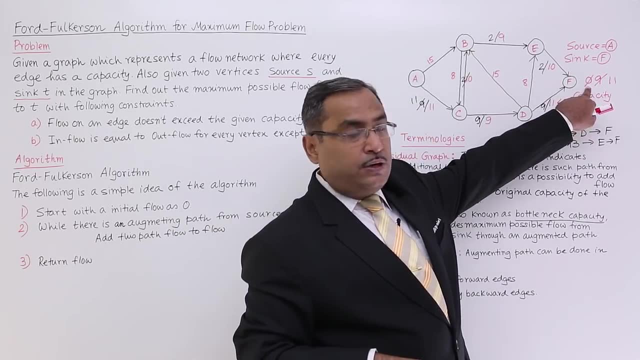 yes, we are getting so many augmenting paths, So here we have demonstrated two of them. Then at this path flow to flow. So this path flow should be added with the flow. So initially it was zero Then. 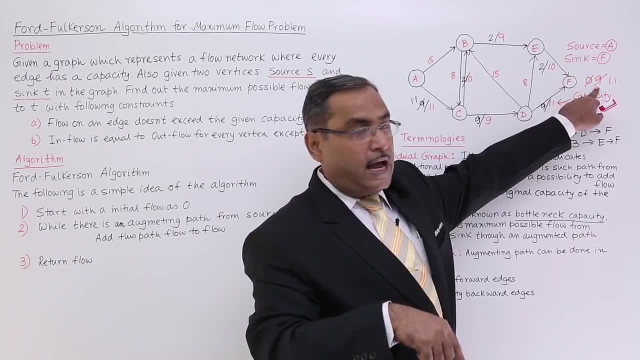 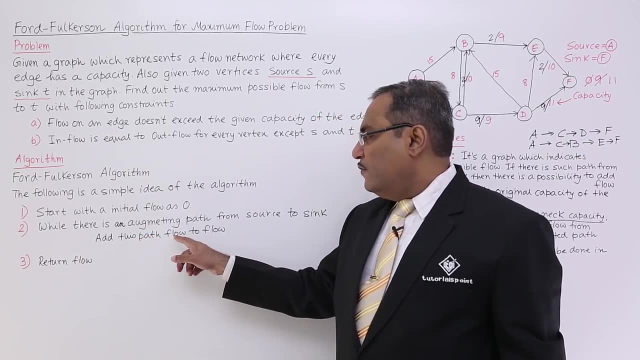 I allowed flow of 9.. So it has become 0 plus 9,, that is 9.. And then I allowed 2 through this, So 9 plus 2,, that is 11.. So now just add this path flow to the flow value And in this way, 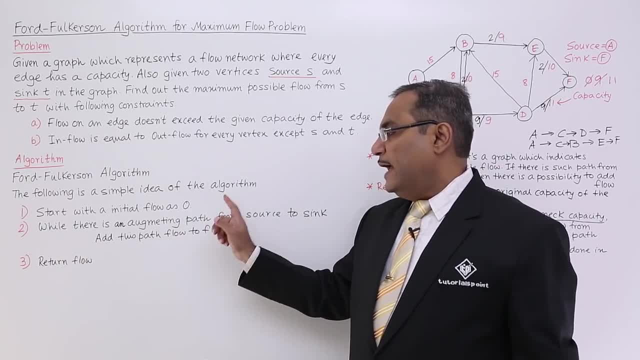 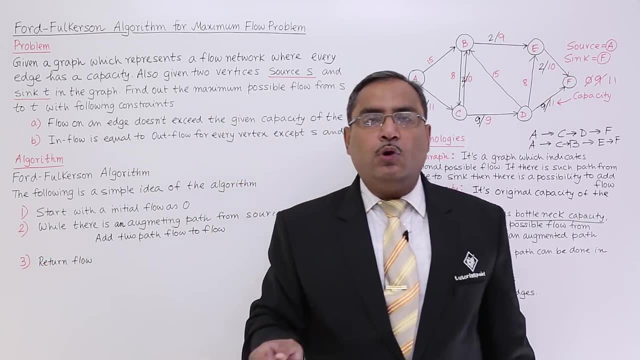 we are going to do until there is no augmenting paths are possible, from source to target, source to sink, And after doing this, the value of the current flow will be returned, And that is the maximum flow of the network. In this way the algorithm will work. Please watch. 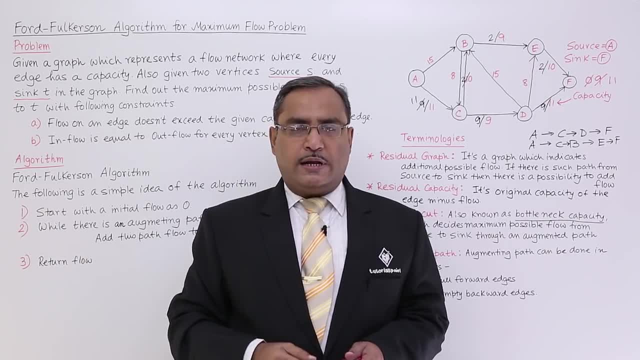 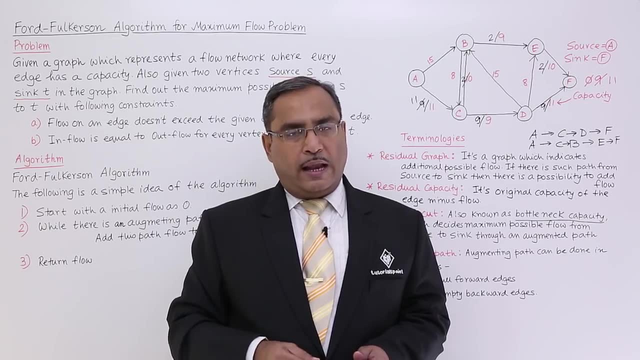 the next video where we will be going for one example for the better and crystal clear conception, to generate the crystal clear conception and better understanding on this particular algorithm. So that video will be in the continuation of this one. Thanks for watching this video.